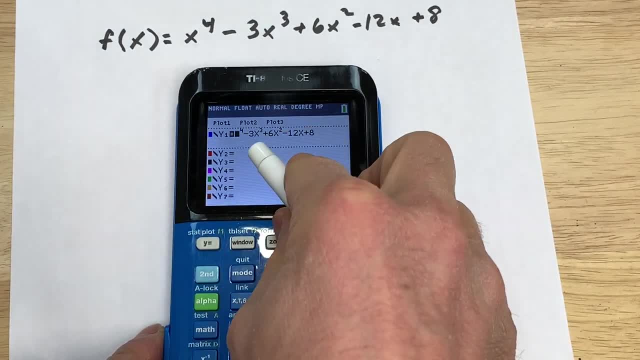 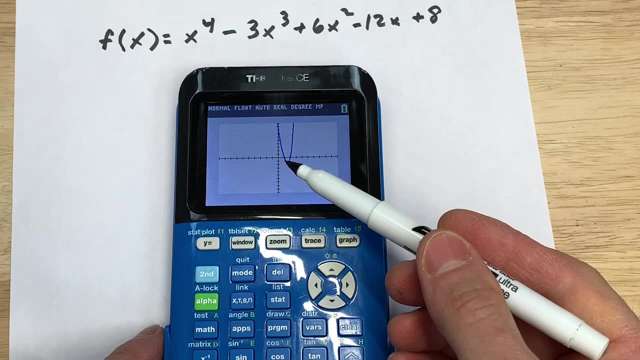 want to input that polynomial in for y1.. So then what we're going to do is we're going to go over here to graph and you can see that it's crossing the x-axis at 1 as well as at 2.. So let's just make. 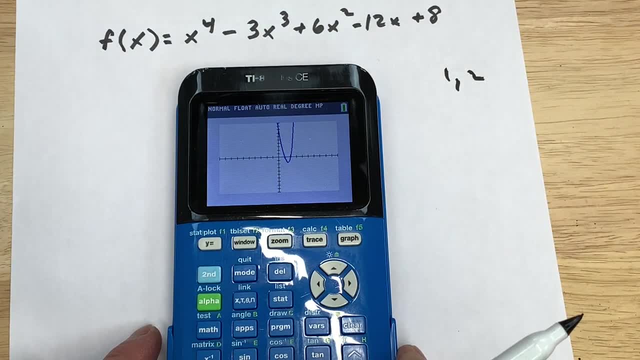 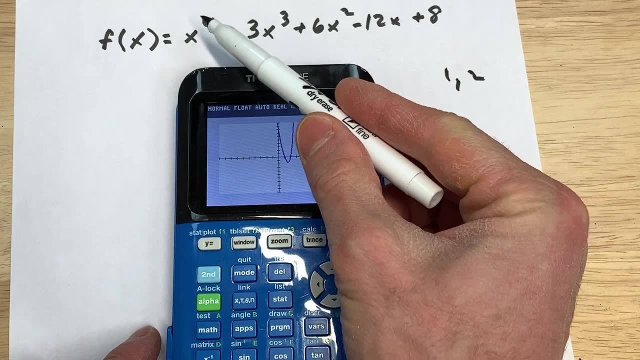 a note of that 1 and 2 are what are called zeros of our polynomial meaning: when x equals 1, y equals 0.. When x equals 2, y equals 0.. But you can see, this is a fourth degree polynomial, which means: 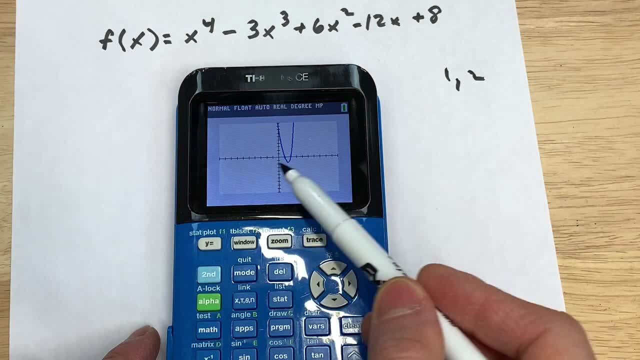 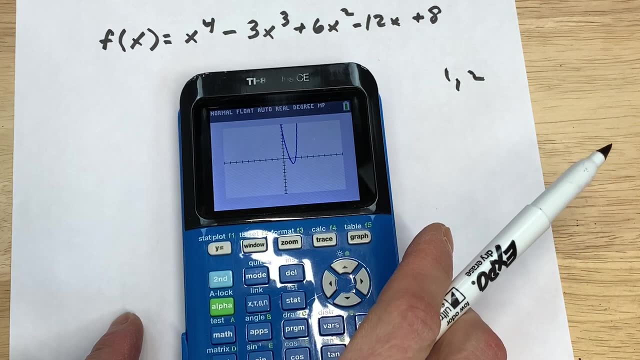 that there's going to be four zeros, But you can see that two of them are going to be imaginary, because it's not crossing the x-axis four times, It's only crossing at two points. How do we find all of the zeros? Well, we know that 1 and 2 are zeros. Let's go ahead and do some synthetic division. So if 1 is, 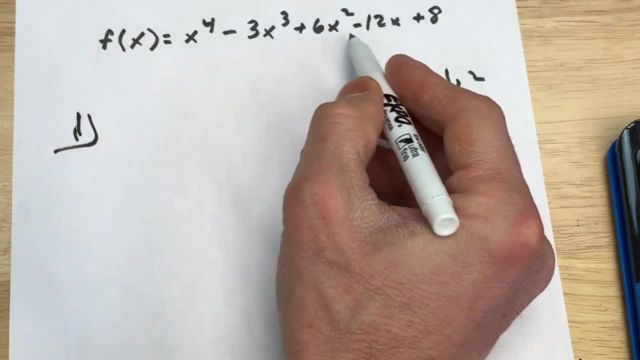 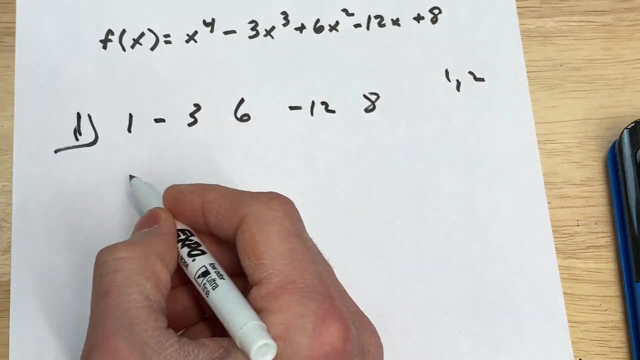 a 0,. let's put the coefficients of our polynomial here: 1, negative 3, 6, negative 12, 8.. You can see there's no missing terms. so we don't need to put a 0 for a placeholder. We bring down that. 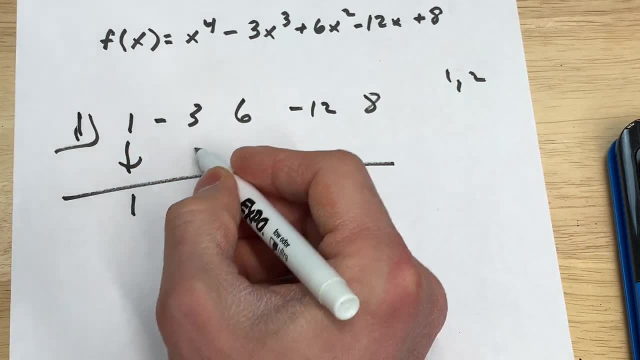 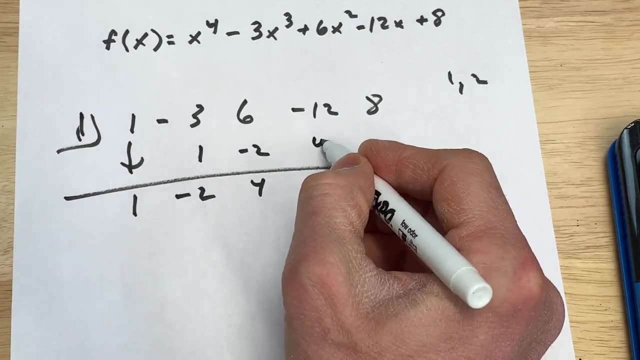 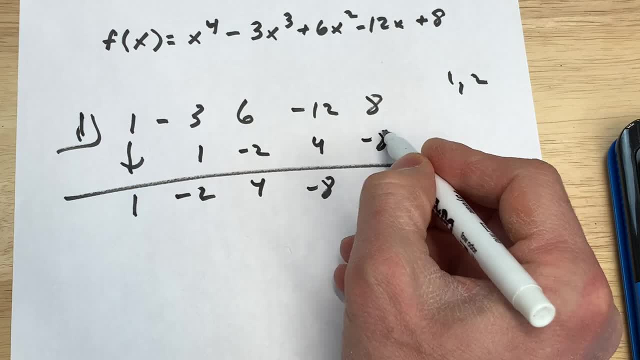 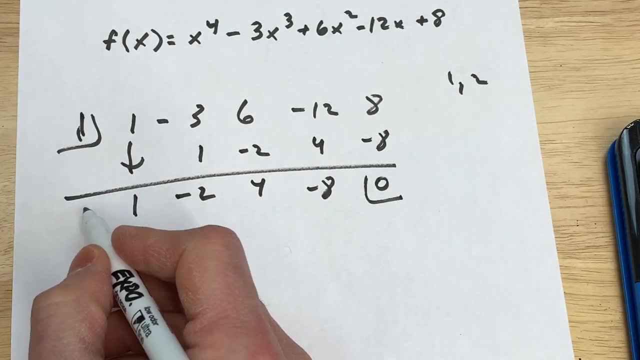 Now you can see you're getting 0 here, which tells us that 1 is a 0. And what we can do? now? we also know that 2 is a 0. Let's go ahead and do synthetic division with 2.. So what we can do is we can again. 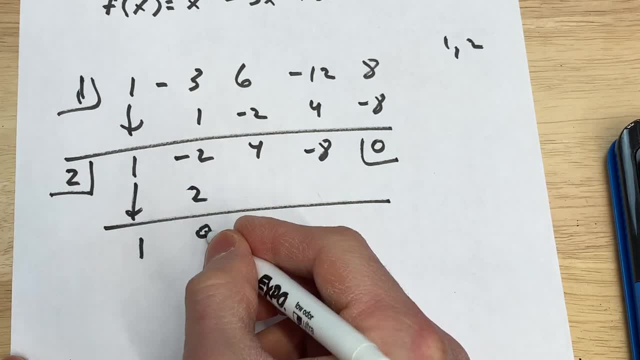 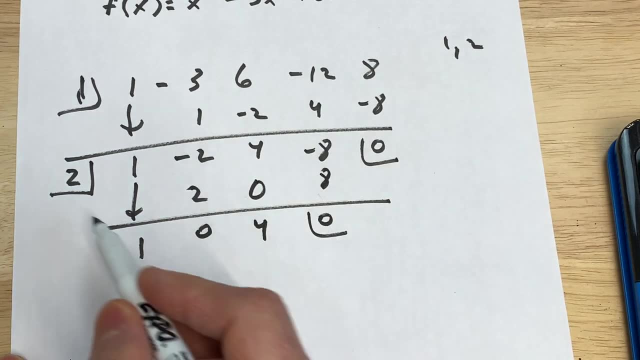 bring down that first term: multiply on the diagonal- add straight down. multiply on the diagonal- add straight down. multiply on the diagonal- add straight down. Now you see how we're getting 0 again. so we know that 2 is a 0. And we started with x to the fourth and we're going to do that. 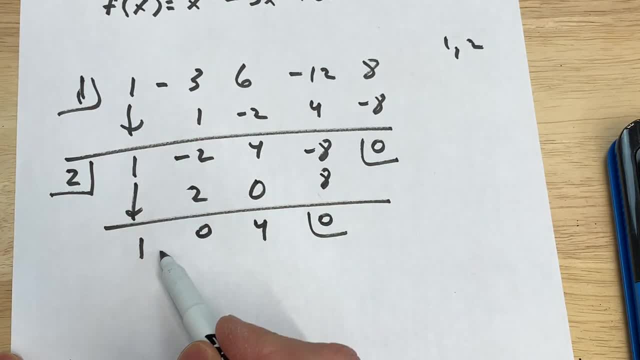 every time we do the synthetic division It goes down by 1 degree. so it's x cubed. Now it's x squared. So what we have here is 1x squared plus 0x plus 4.. And if we set that equal to 0,. 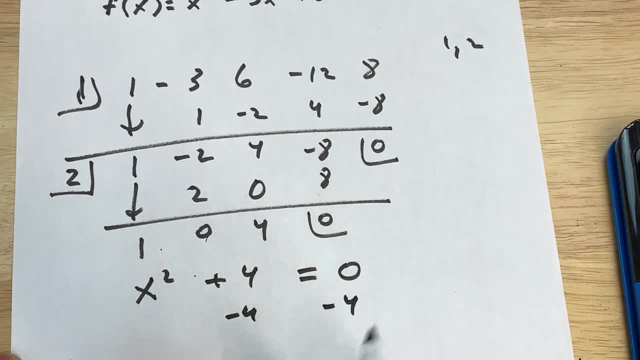 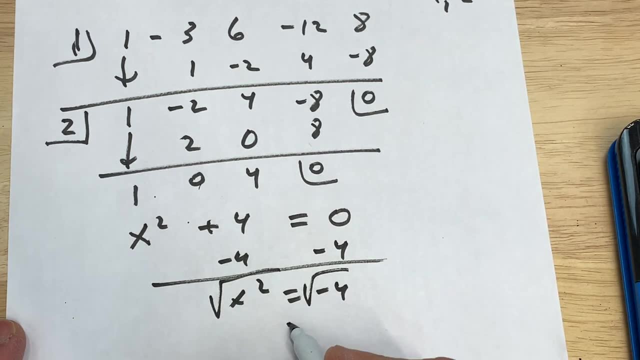 we can find the remaining 0.. So I'm going to subtract 4 from both sides and that's x squared equals negative 4.. I can take the square root of both sides. Remember when you do that you get two answers plus or minus. Square root of 4 is 2.. Square root of the.